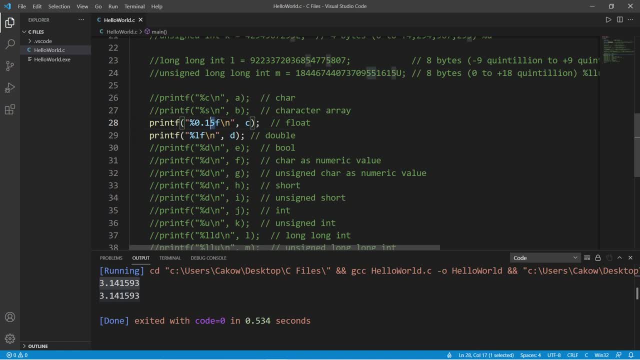 and the amount of digits I would like to display. So I would like to display 15 digits after my decimal, And I'll do that for my double as well. So after the percent sign 0.1f, then add lf And 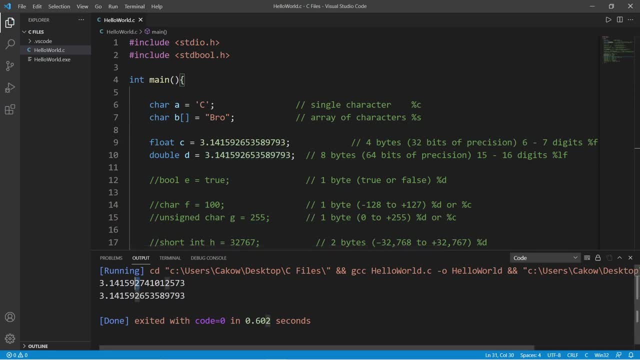 let's take a look at these numbers. Okay, after my two, which is, I believe, the sixth digit after the decimal, we actually look at the number of digits that I would like to display. So I'm going to display two and then add 0.1f, So this is actually the same number. I'm going to display this number if I want to display. 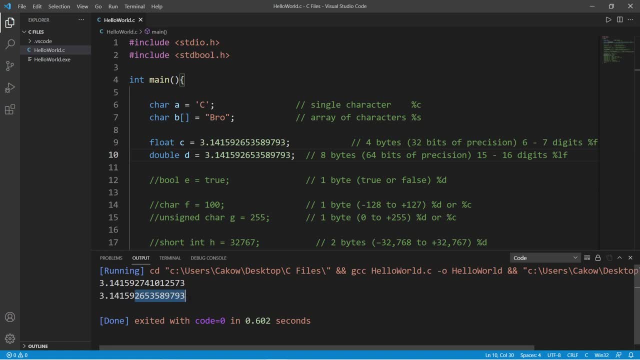 the difference, And then I'm going to apply a double here. At this point we'll actually losing our precision. These numbers are not the same, But our double will actually retain these numbers. So, point being, a double is even more accurate than a floating point number. there is more precision, but it uses 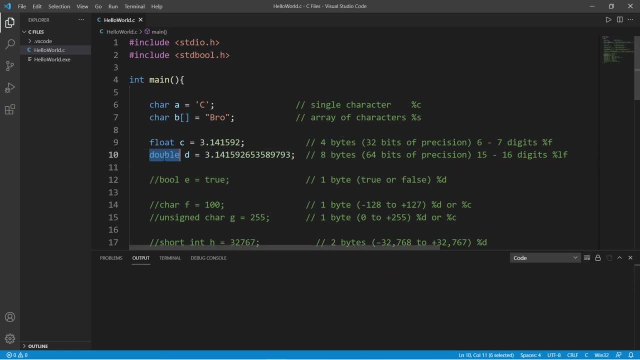 more memory. a double uses eight bytes of memory. Because of this reason, we tend to use doubles a lot more than floats, just because they're more precise. We don't want to lose our precision. Next up we have booleans to work with booleans and see include this at the top: std booleh booleans store. true or false? 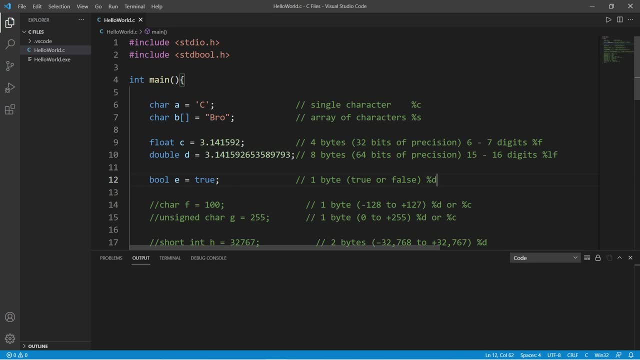 data false. So they work in binary 1 represents true and 0 represents false. So when you need to declare a boolean variable, you type bool, then a variable name and you set it equal to true or false. Technically we only need one bit. 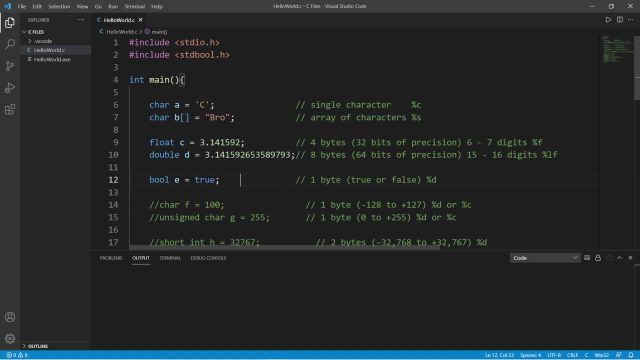 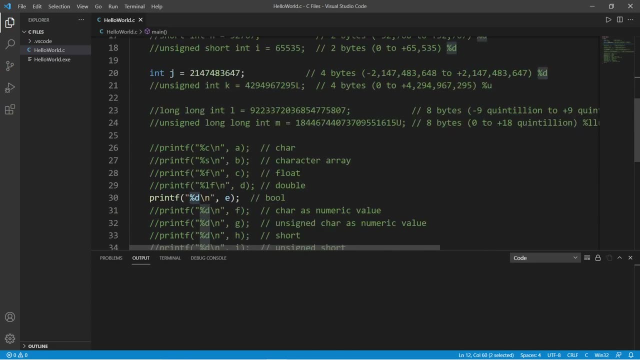 to represent true or false- 1 for true and 0 for false, but this still uses up one byte of memory. And then to display a boolean, you can use %d. So if I was to display this boolean variable, I would use %d, So 1. 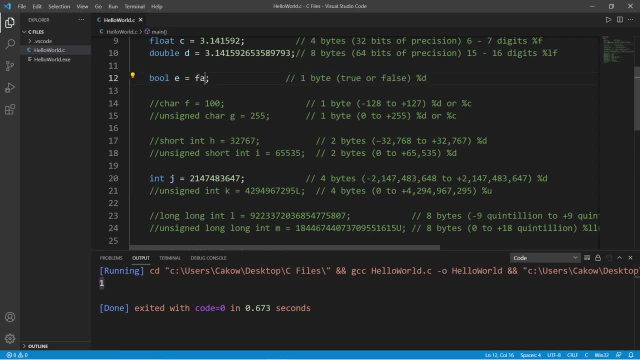 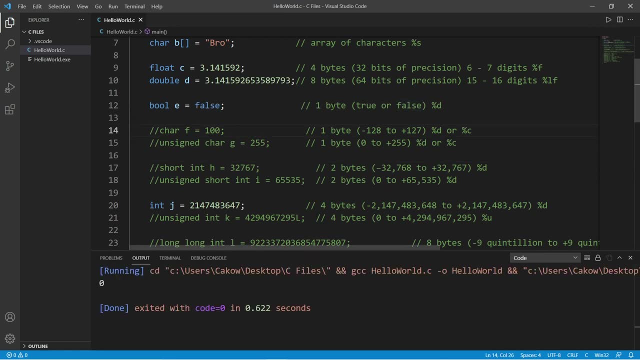 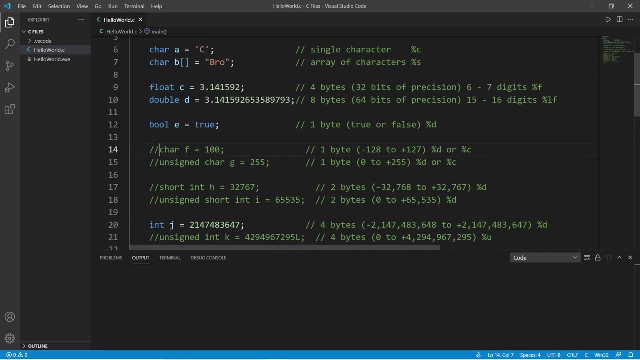 corresponds to true and 0 corresponds to false, Although there are some tricks that we can do in the future where we could display the word true or the word false, But for now we're going to stick with %d as the format specifier. So these work in binary: 1 for true, 0 for false. Now another thing. 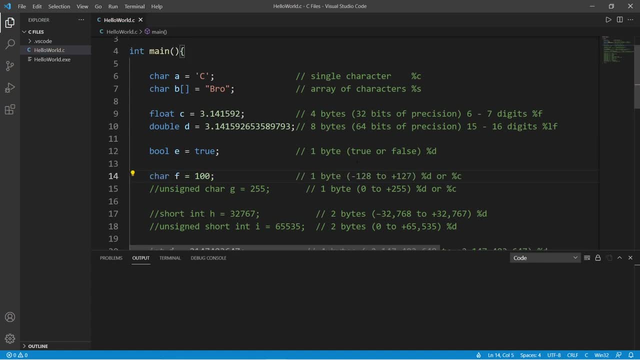 that we can do with chars is that we can store a whole integer between the range of negative 128 to 0.. To positive: 127.. So in this example we have char f and I will store the integer number 100.. We can display this number as either a decimal, an integer or a. 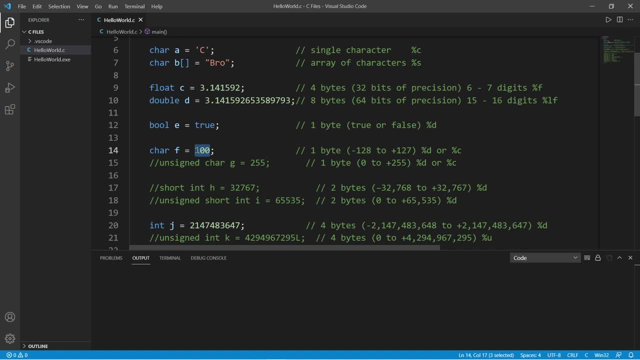 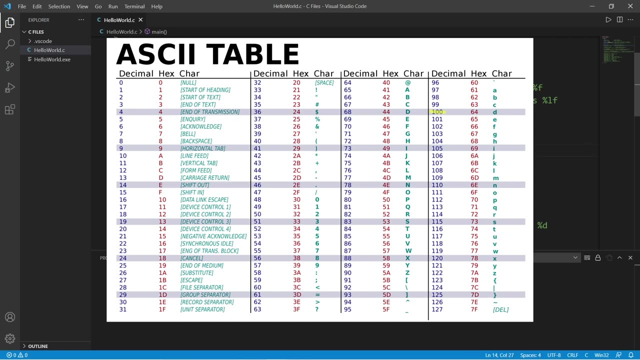 character. So if I was to display this number as a character, we will use the ASCII table to convert this number to a character representation. The ASCII table has a range between 0 to 127.. So if I was to display this number as a decimal, 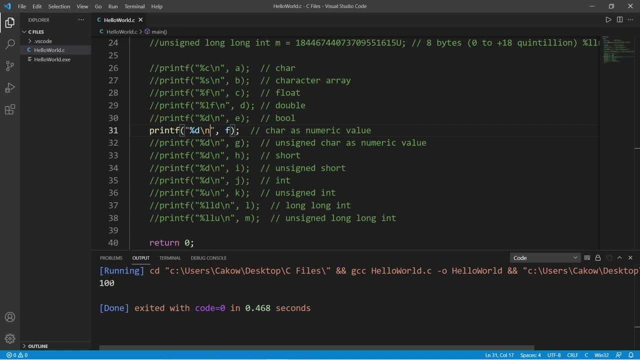 using the %d format specifier, of course this will display as 100.. But if I was to convert this to a character using the %c format specifier, this has a corresponding character and that would be lowercase d. So I'm actually going to change this to something else. What about? 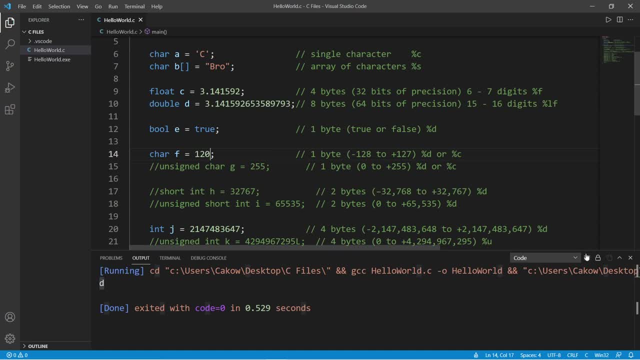 I don't know 120.. So let's see what the character representation of that number is. And that would be a lowercase x, So you can use chars to store more than single characters. You can also use them to store a whole integer. However. 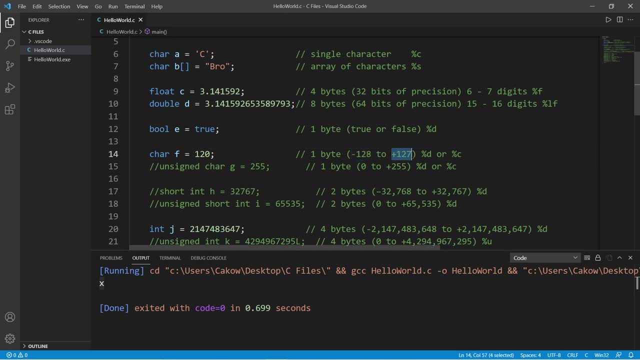 However, the range is between negative 128 to positive 127, because they have one byte of memory. Now there is a keyword unsigned, So when you declare a variable that is unsigned, we disregard any negative numbers So effectively. this doubles our range with our positive numbers. 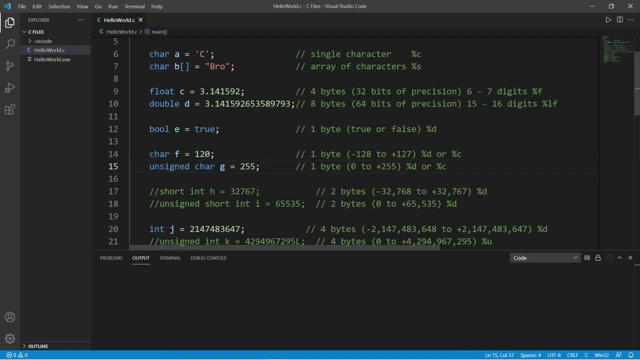 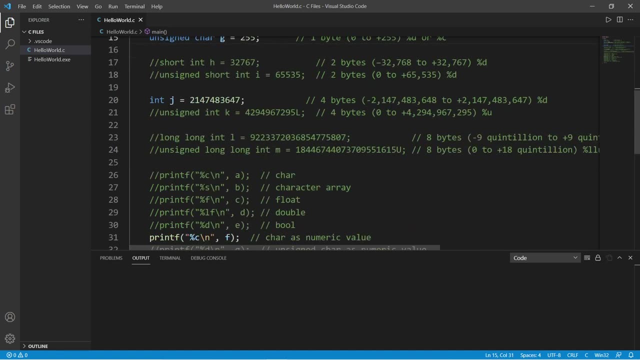 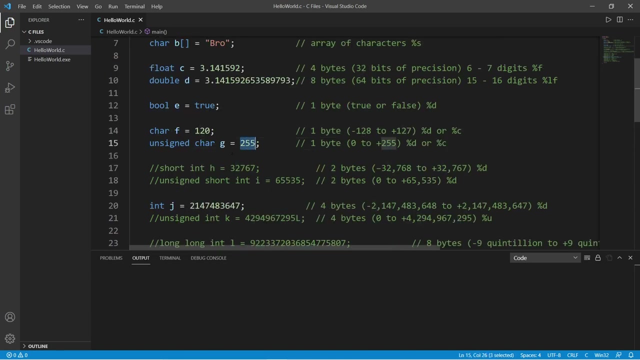 So if we have unsigned char, we can store a number between 0 to positive 255, because we know we're not going to store a negative number. So then, if you need to display an unsigned character, we can use just %d. I'm going to store 255 within my unsigned char, and that would be, of course, 255. 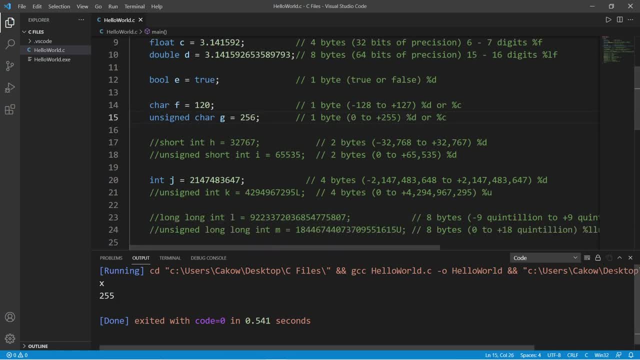 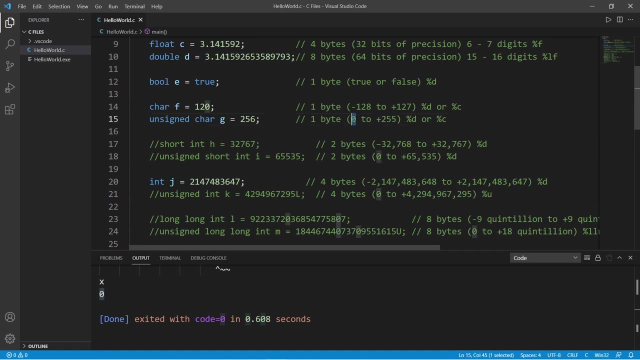 However, if we go beyond this range, this will overflow and go back to 0. So if I was to display this, we have a warning: Unsigned conversion from int to unsigned char, So then this resets back to 0.. So if you go beyond the maximum range, this will reset all the way back to 0. 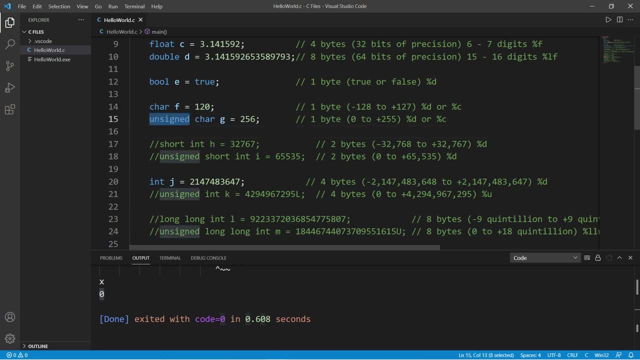 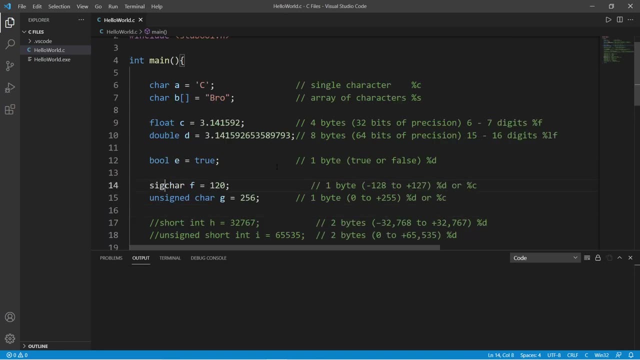 Whatever, the beginning is. So if you add this keyword unsigned, you can effectively double the range of positive numbers that you can store within a variable. By default, most data types are already signed, but we don't need to explicitly type that. So, point being, with chars you can store more than a single character. 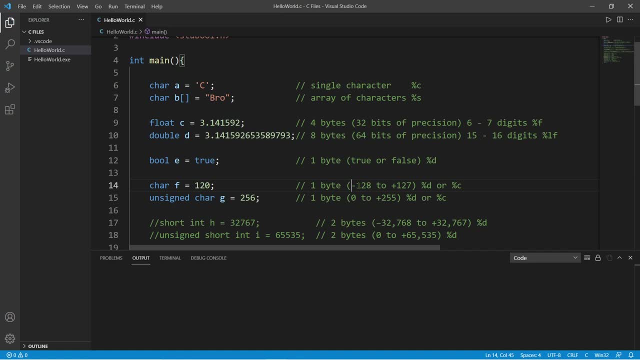 You can store a whole integer between ranges negative 128 to positive 127 if it's signed. If it's unsigned, you can store numbers between 0.. to 255.. You can display them as an integer by using the %d format specifier. 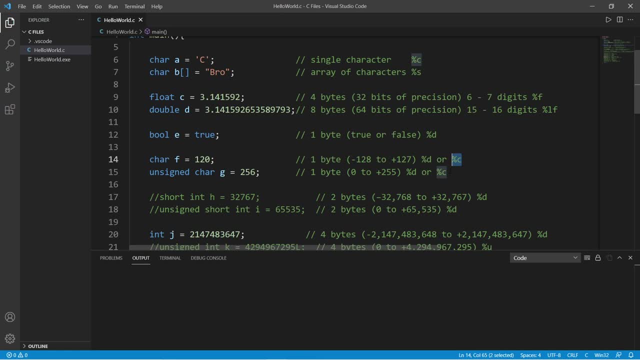 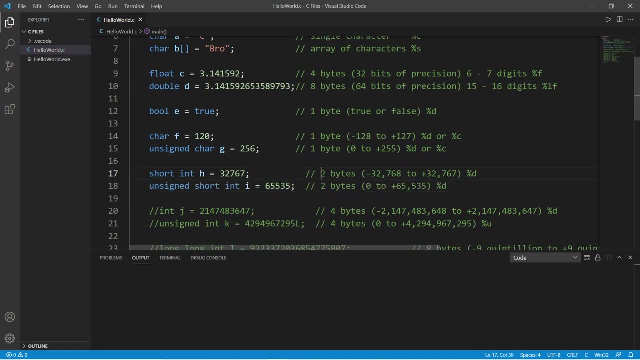 or you could convert them to a character using the ASCII table by using the %c format specifier. Next, we have short ints. Short ints use two bytes of memory. They can store a number between negative 32,768 to positive 32,767,. 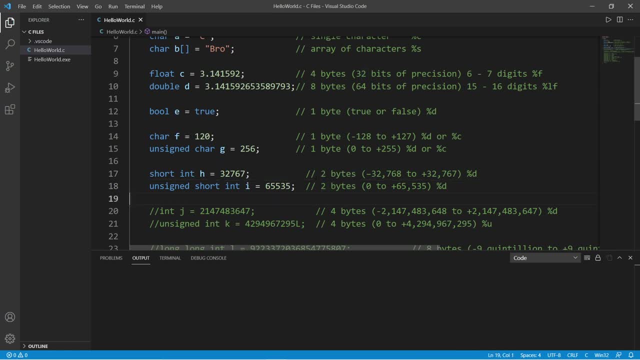 because, well, they use two bytes of memory. They can only store a number so large, And if it's an unsigned short int, the range is instead between 0 to 65,535.. And we use the %d format specifier to display a short int. 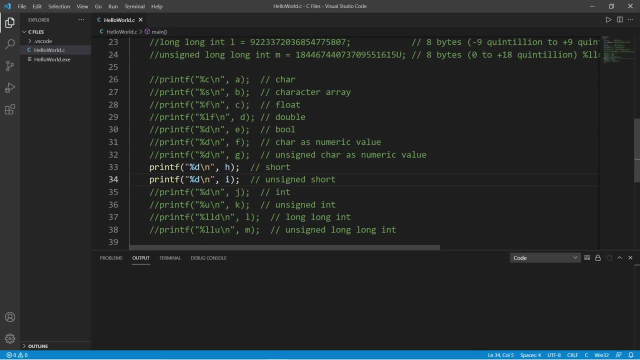 So within my printf statement I'm going to display these two numbers. So I will display variable h and i. h is a short integer and i is an unsigned short integer. So these are the maximum values for a short integer and an unsigned short integer. 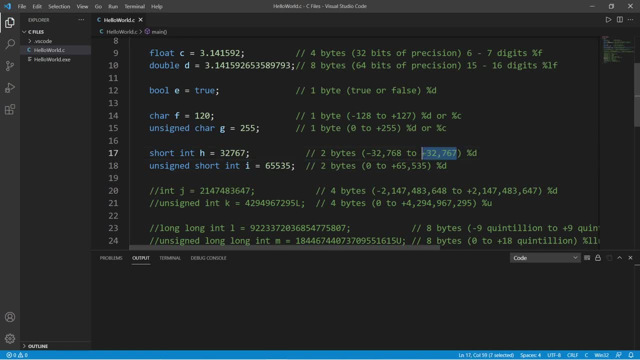 And, like I said, I'm going to display a short integer and an unsigned short integer And, like I discussed with chars, if we go beyond this range we will encounter an overflow. So I'm going to change this short int to 32,768.. 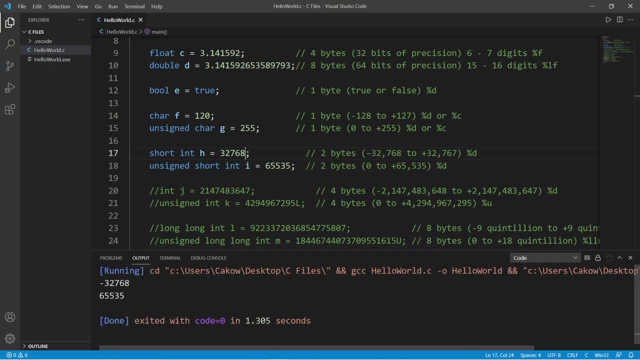 And let's see what number displays. So this will overflow and reset this value back to the minimum value, which in this case is negative 32,768.. And if you do the same thing with the unsigned short integer, that would be 0, because that's the minimum value. 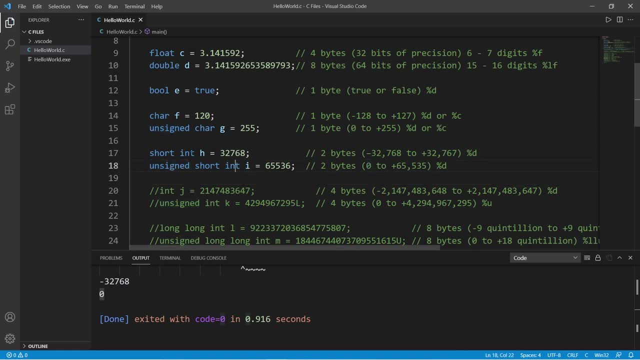 For a short integer, the minimum value is 0.. So if we go beyond this range, we will encounter an overflow. an unsigned short integer. So those are short integers. They use two bytes of memory and they can store numbers between these ranges, depending if it's signed or unsigned. Oh, and another way. 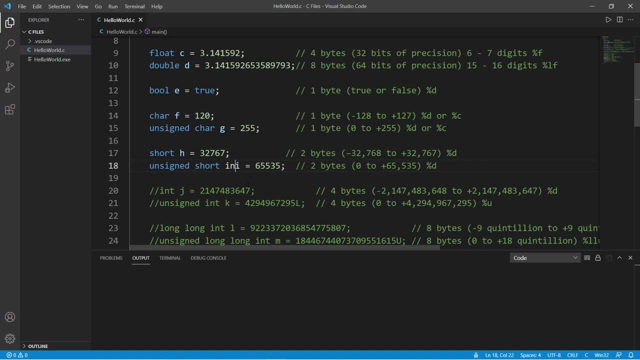 of writing these. you don't necessarily need to declare these with the word int. You could just say short, and that would do the same thing. People usually just call them shorts instead of short ints. So those are what shorts are Now with integers. we kind of discussed this in the last. 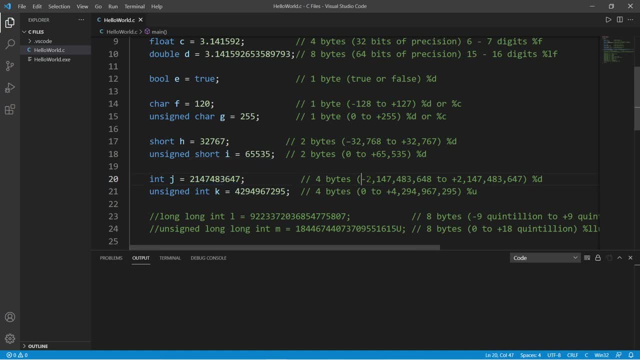 video. just briefly, Integers store a whole number between just under negative 2 billion to just over positive 2 billion, because they use four bytes of memory and we use the %d format specifier to display a signed integer. If that integer is unsigned, the range changes from zero to just. 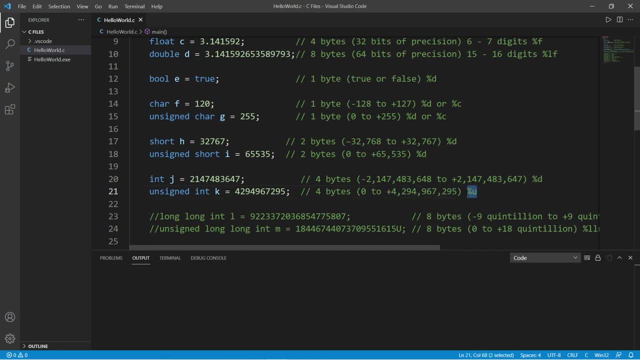 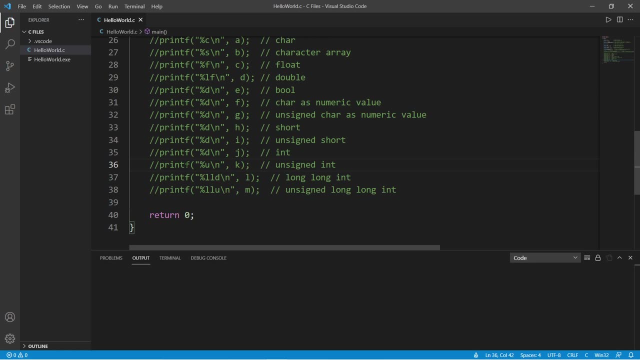 over positive 4 billion. However, there is a different format specifier To display an unsigned integer. you instead use %u. So then let's display these: %d for a signed integer and %u for an unsigned integer. And these are the maximum numbers. And then, if I was to exceed the range, 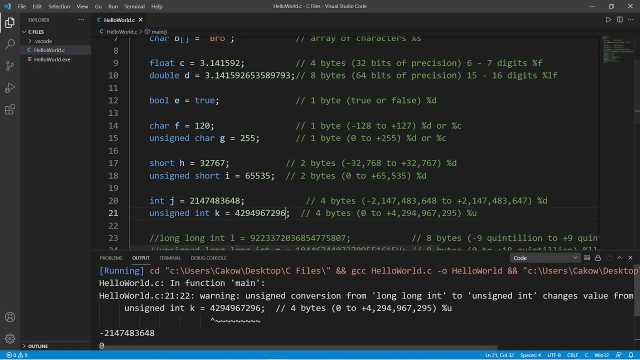 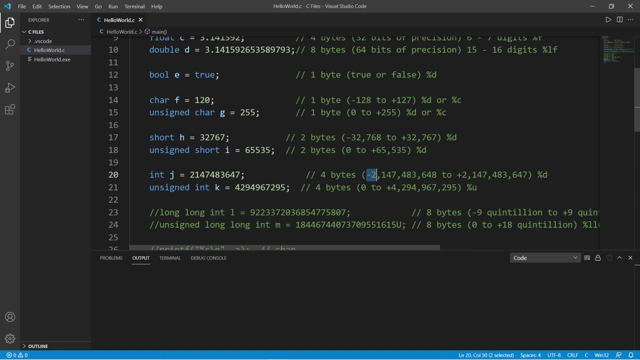 this again would cause an overflow and reset these numbers back to their minimum values. So those are standard integers. They use four bytes of memory so they can store numbers between these ranges, depending if they're signed or unsigned. So those are standard integers. 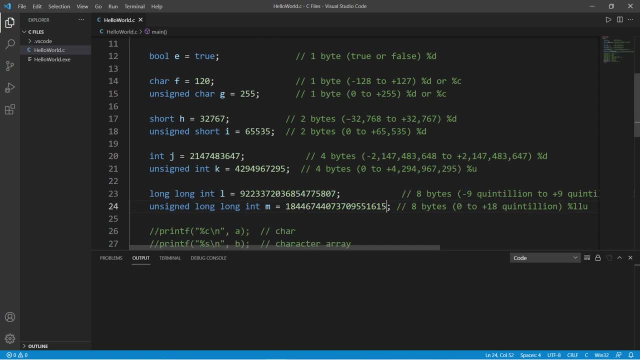 All right, the last data type we're going to talk about for this topic is a long, long integer. Now, the reason that we have long twice is that with standard integers these are already considered longs, but we don't need to explicitly type long for standard integers So to represent a really 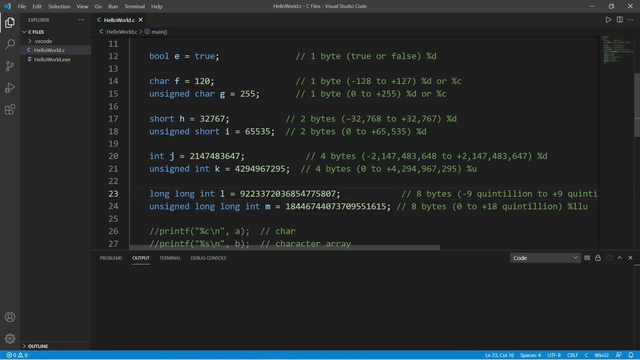 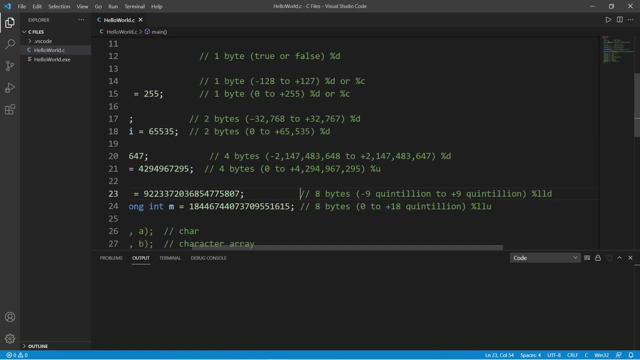 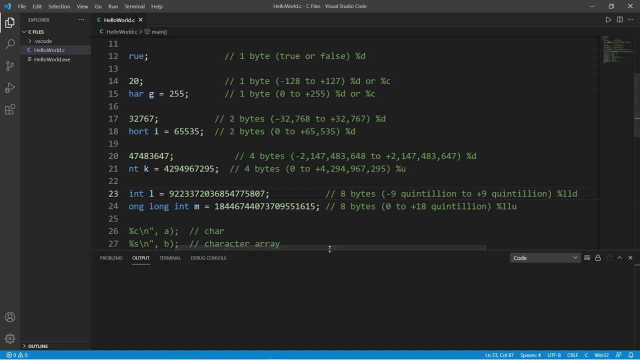 large number, we can use a long, long integer And these use eight bytes of memory. The effective range for a signed long, long integer is just a long, long integer. So we can use a long, long integer. So that's underneath 9 quintillion to just over 9 quintillion And the format specifier for a long 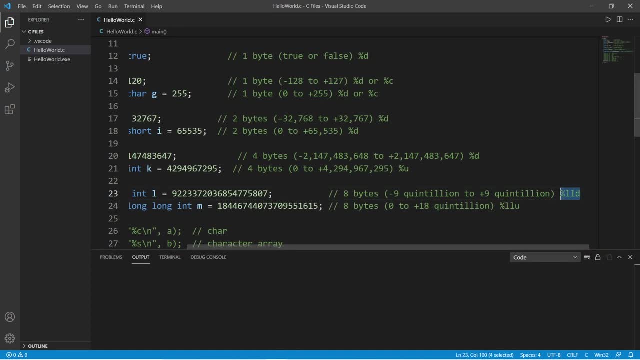 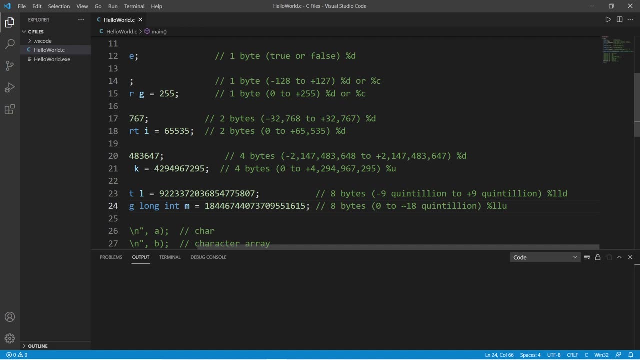 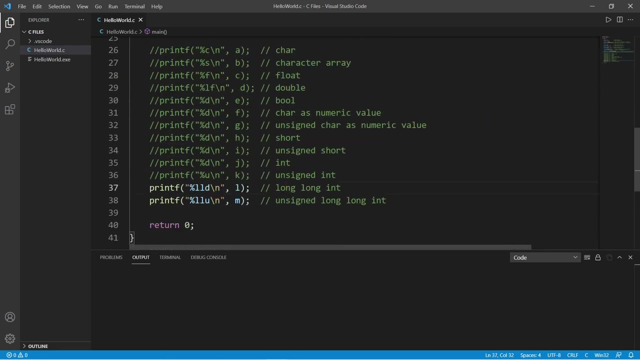 long integer, one that is signed is %lld. Now, if it's unsigned, that changes the range between zero to just over positive 18 quintillion And the format specifier is %llu, Then let's display these. So, for a signed long, long integer, that is lld, And if it's unsigned, that is %lld. 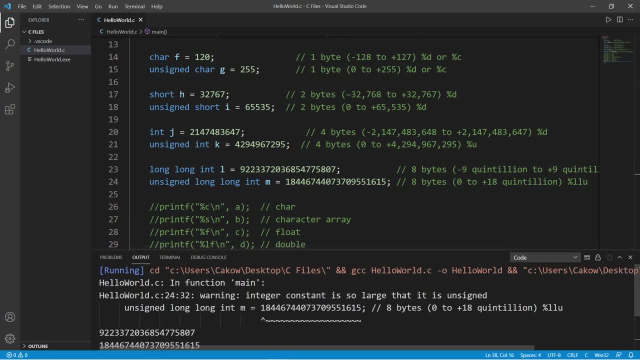 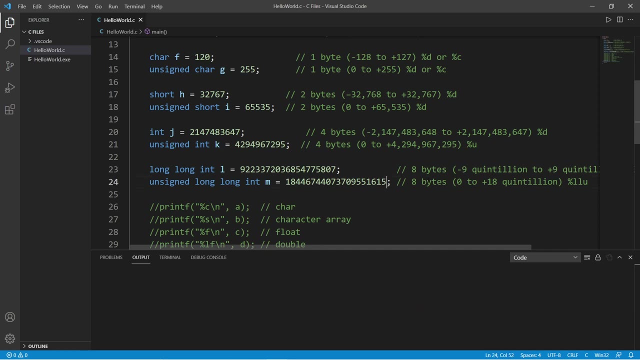 Now we'll encounter a warning. So this warning applies to our unsigned long, long integer. Integer constant is so large that it is unsigned. So one way in which we can prevent that warning is, after our number within our unsigned long, long integer, add a u to the end of this. So then we